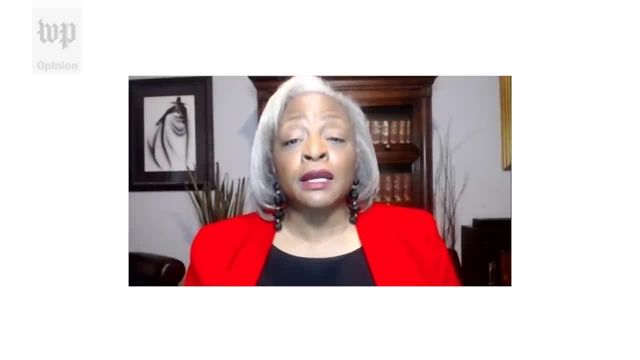 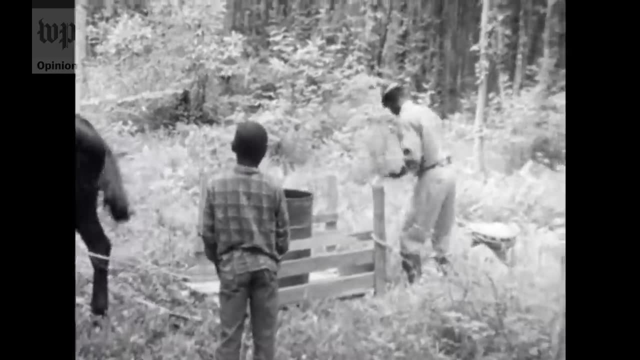 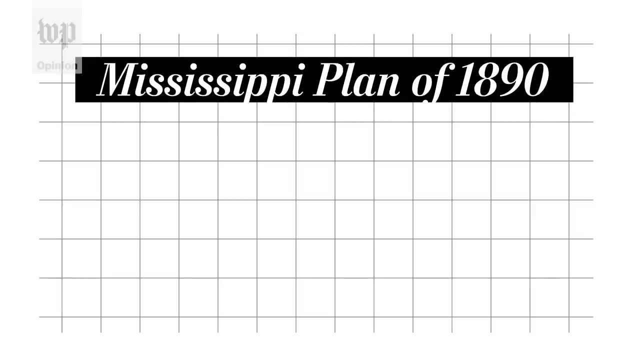 What Mississippi did was Mississippi said: we will take the societally imposed conditions on African Americans and use those conditions as the access to that conversation that is white, specifically to the ballot box. Mississippi passed a new state constitution that required every citizen to pay a poll tax. 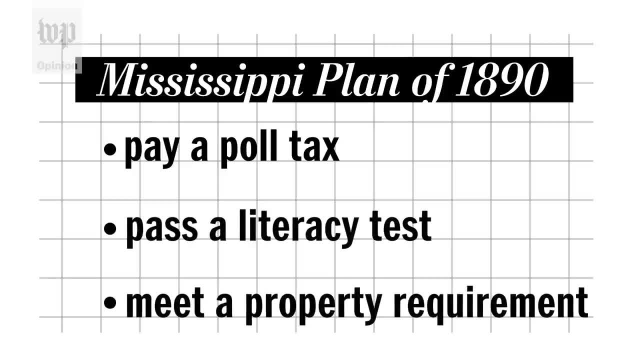 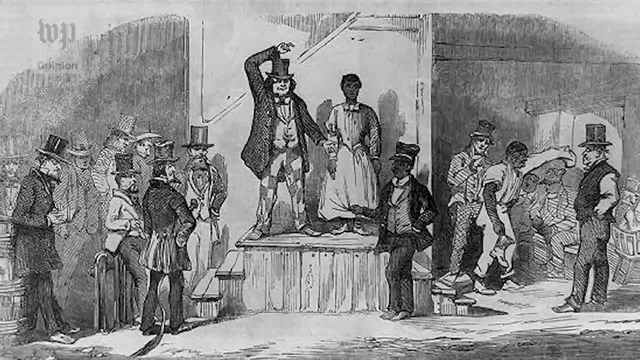 pass a literacy test and, in some cases, meet a property requirement. At the time, Black people were less than 30 years out of slavery when they earned no money and were blocked from reading. The Mississippi Plan of 1890 was applied equally. 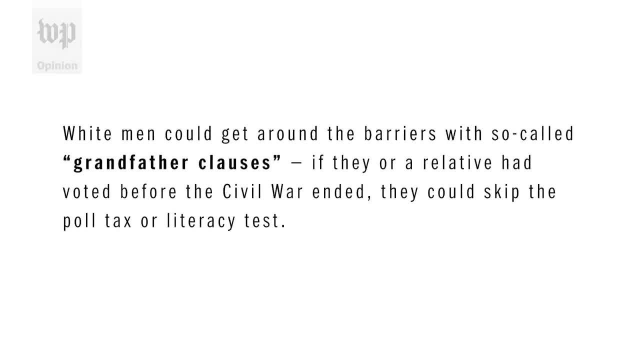 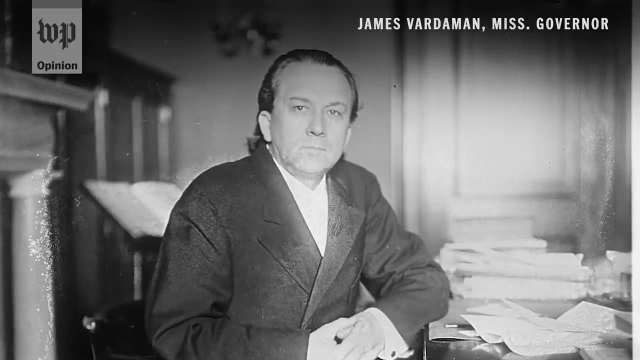 to Black and white voters. but white men could get around the barriers with so-called grandfather clauses. If they or a relative had voted before the Civil War ended, they could skip the poll tax or literacy test. A Mississippi governor later admitted the provisions had no other purpose. 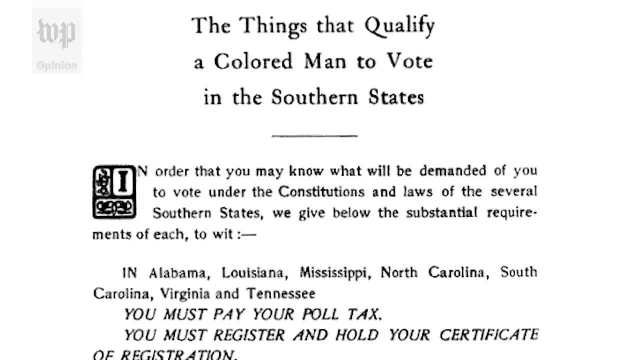 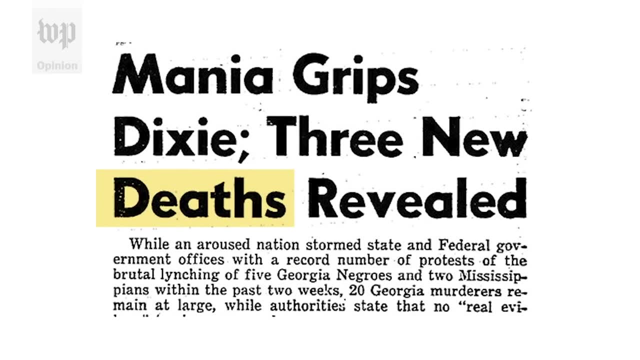 than to eliminate Blacks from politics. That's how a blueprint to circumvent the 15th Amendment was created and other states followed Mississippi's lead. In the Jim Crow era, Black voters were often met by violence. Civil rights workers who helped other African Americans. 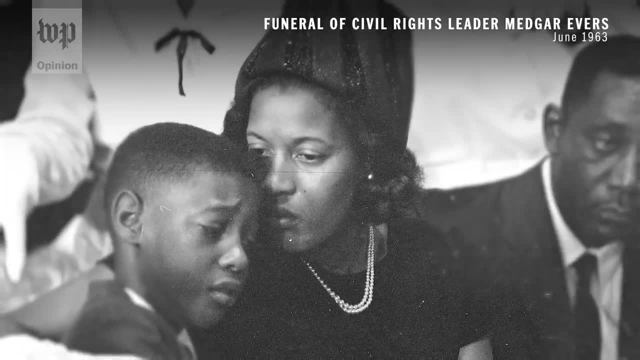 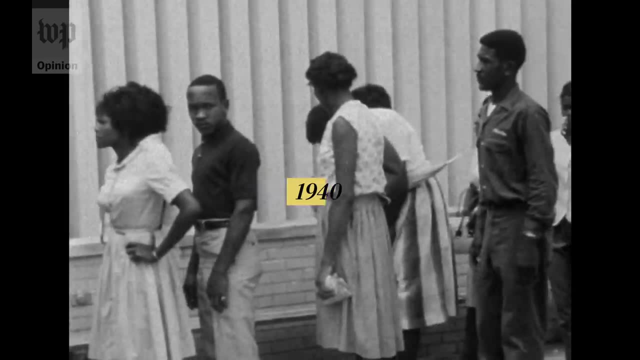 to vote were shot, lynched or violently harassed by vigilantes and police, And even though the 19th Amendment passed in 1920 to give women the right to vote, by 1940, only 3% of eligible African Americans. 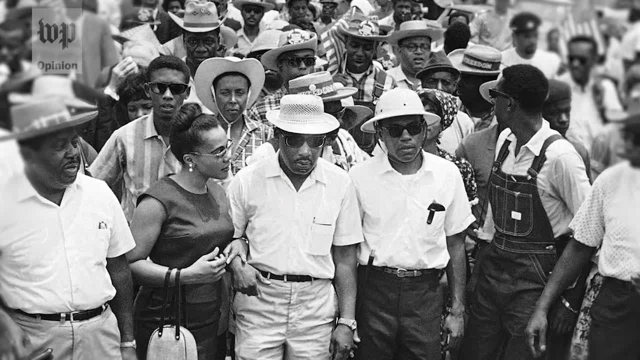 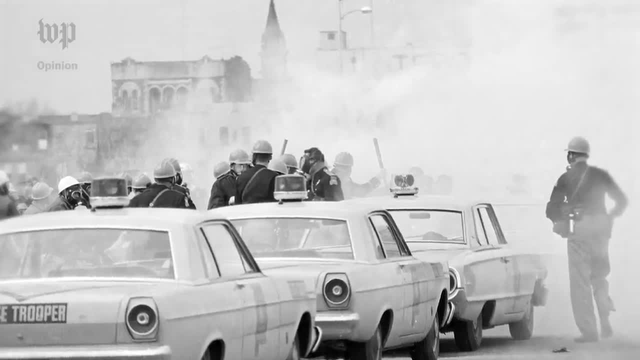 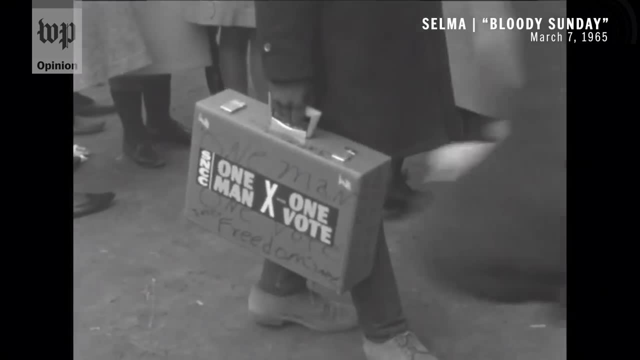 in the South were registered to vote. The Civil Rights Movement is one of those moments in American history where the US feels a depth of pride because it overcame. it overcame something as villainous as Jim Crow, And it took a lot of bodies. 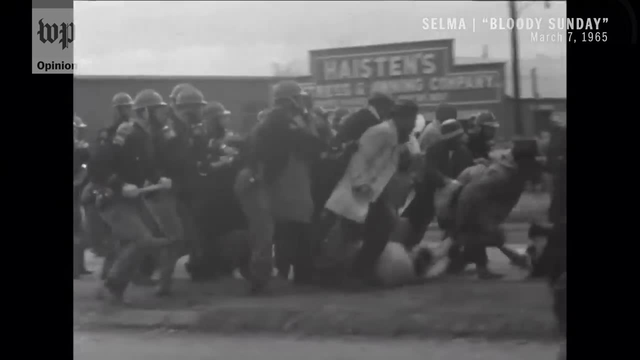 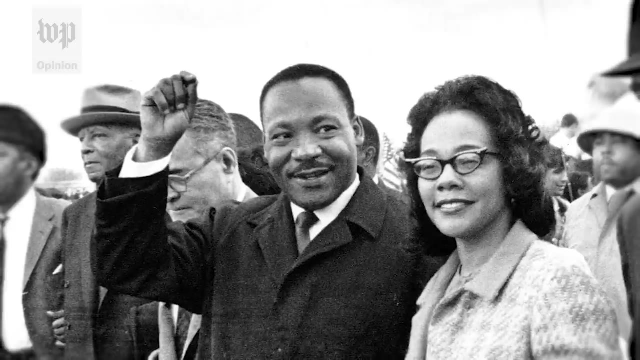 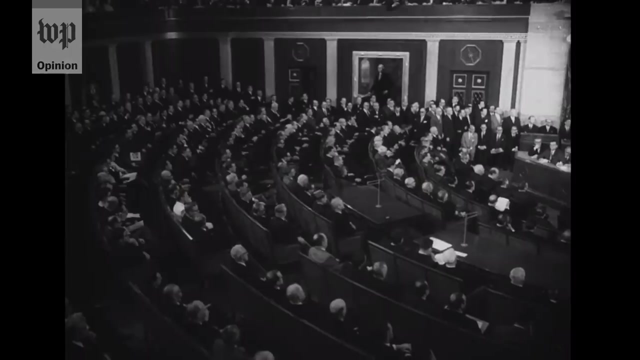 It took this kind of moral power of the nonviolent movement. It took grassroots organization and mobilizing. It took Martin Luther King, This hard-earned legislative victory of the Civil Rights Act of 1964, the Voting Rights Act of 1965.. 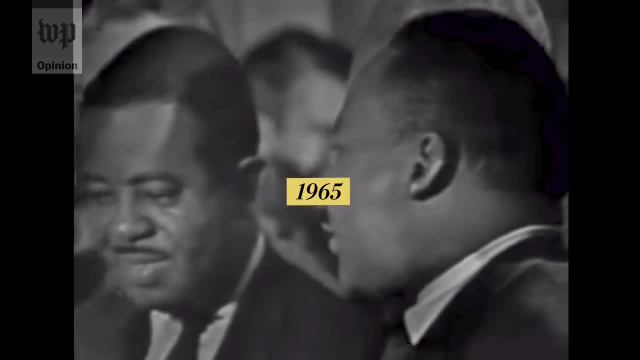 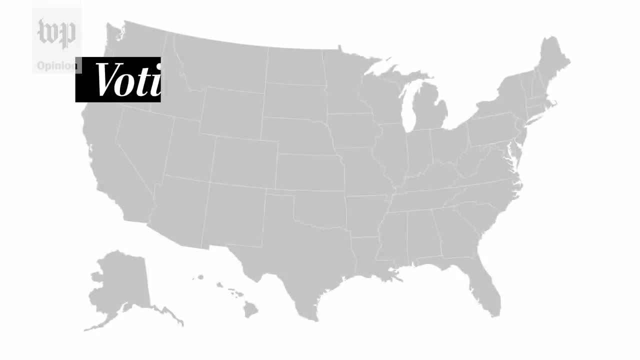 The Voting Rights Act was hailed as a defining civil rights legislation of its time. It was especially important because it had an enforcement mechanism. the 15th Amendment lacked Under Sections 4 and 5 of the VRA, states with a history of discriminatory voting laws. 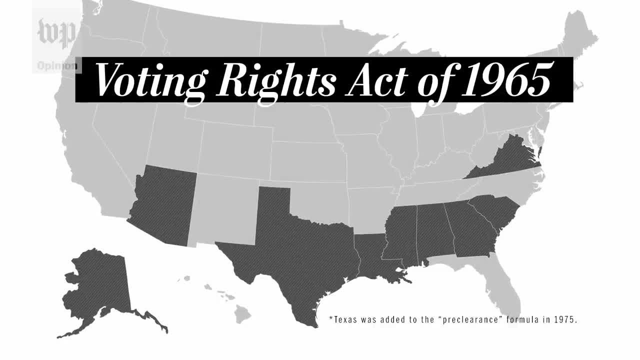 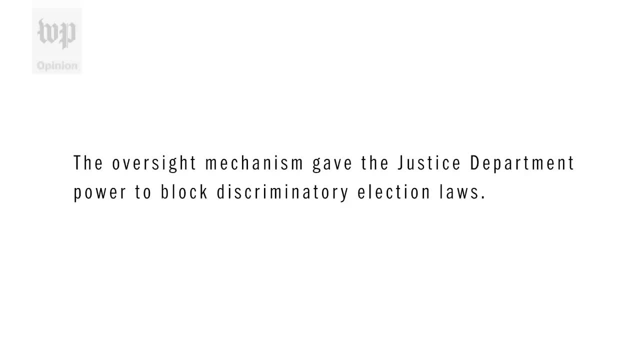 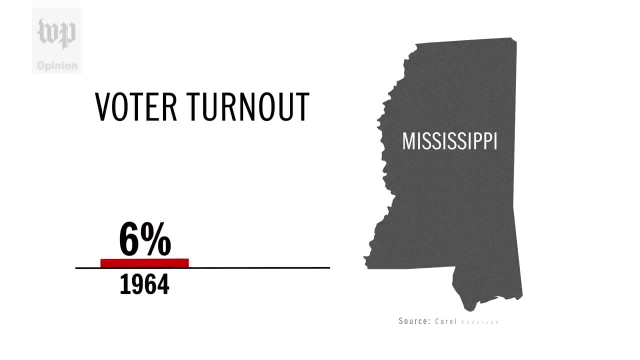 now needed federal approval or preclearance to change their election laws. This gave the Justice Department and federal courts in DC power to block discriminatory election laws. Its impact was profound. In Mississippi alone, voter turnout among Blacks increased from 6% in 1964 to 52%. 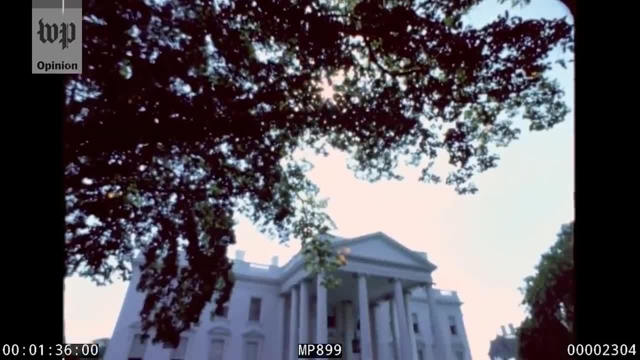 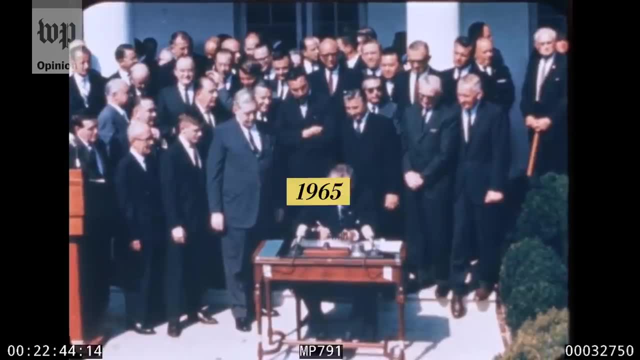 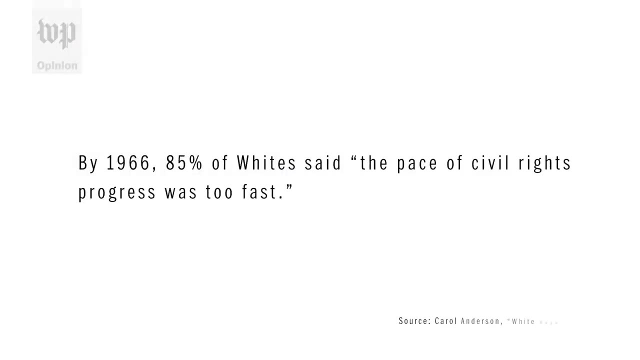 That's 49% in 1969.. By then, President Lyndon B Johnson had established anti-poverty programs to curb inequality. He created Medicare and Medicaid for the elderly and poor and enacted education and housing reforms. By 1966, 85% of whites said: 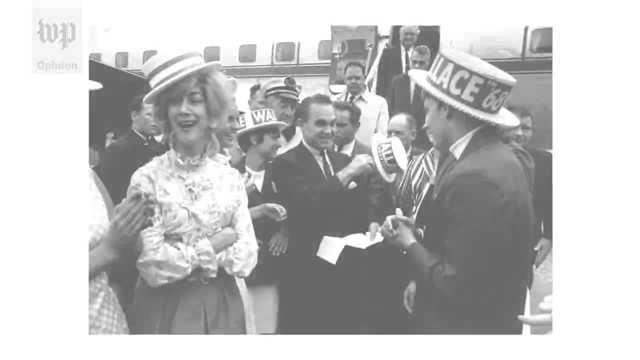 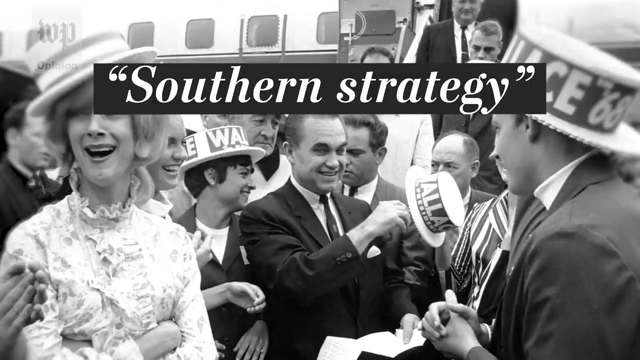 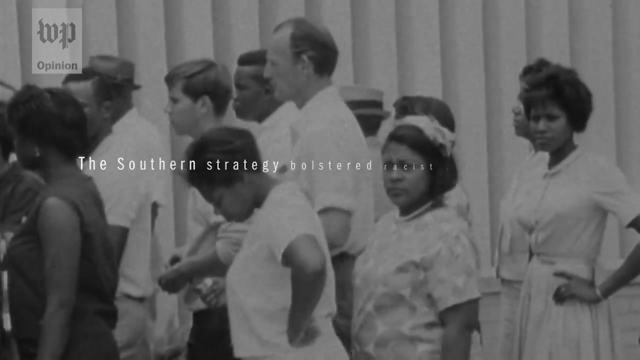 the pace of civil rights progress was too fast And by the 1968 presidential election white resentment had coalesced into the Southern Strategy, Bringing Democrats and disaffected whites into the Republican Party. The Southern Strategy bolstered racist policies and practices without using racist language. 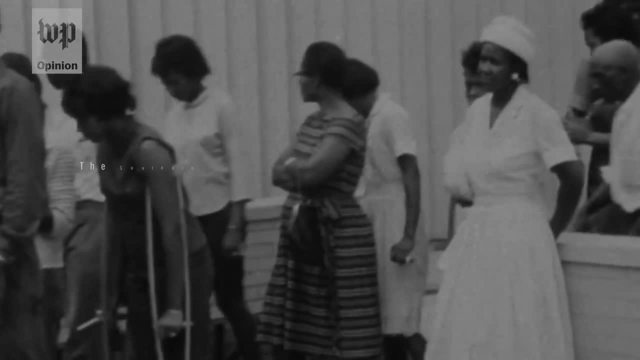 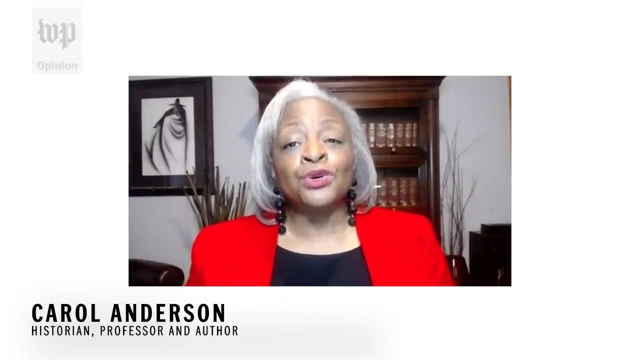 Anderson says this applied to voter suppression as well. Voter suppression is really based on the Mississippi Plan of 1890, where you can't say we don't want Black people to vote. But that's the intent. That's been a key element in the process. 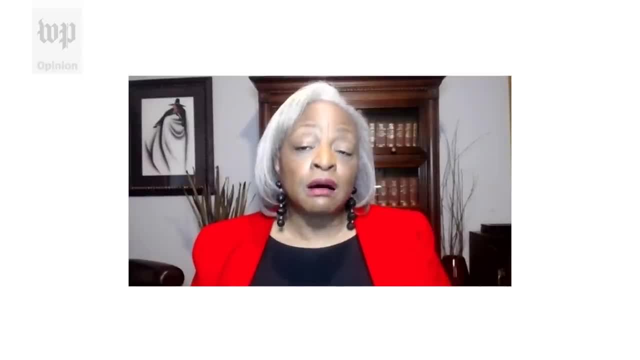 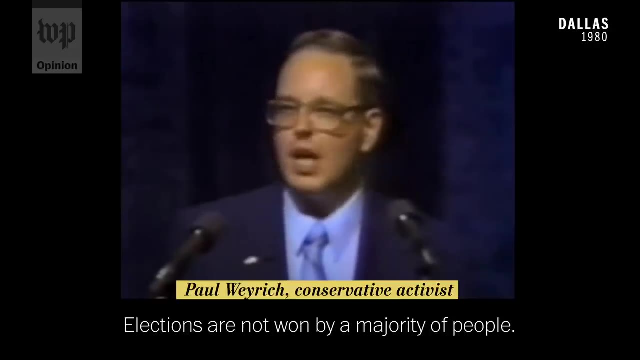 Another key element in the policy of now the Republican Party, I would say another key element in policy- was uttered by Paul Wyrick. They want everybody to vote. I don't want everybody to vote. Elections are not won by a majority of people. 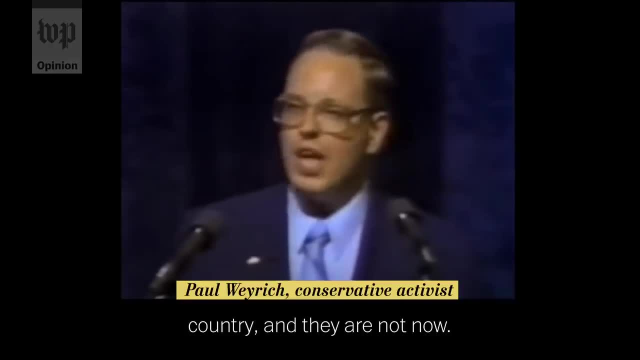 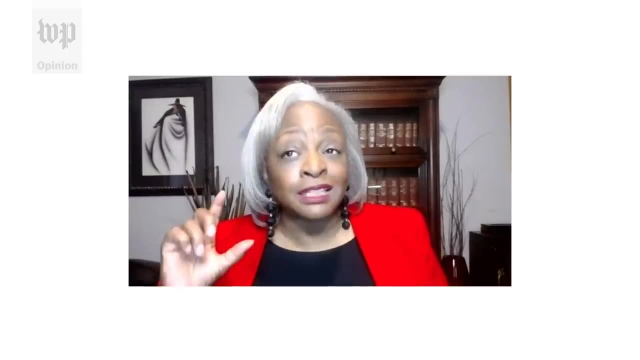 They never have been from the beginning of our country and they are not now. As a matter of fact, our leverage in the elections quite candidly goes up as the voting populace goes down To understand the language of voter fraud and voter suppression that's going on now. that's the framework That our leverage, our power increases when the voting populace is constrained. When President Ford signed the reauthorization of the Voting Rights Act in 1975, the scope of the bill was expanded to protect Latino, Native American and Asian voters. 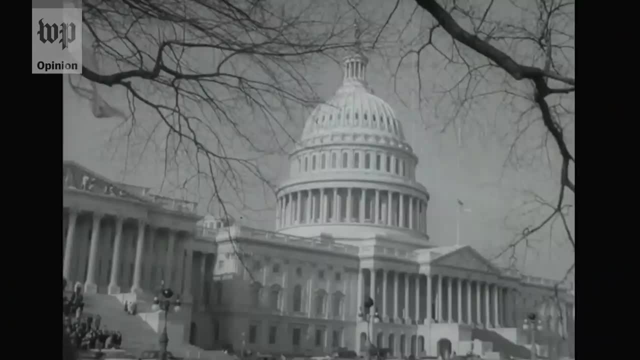 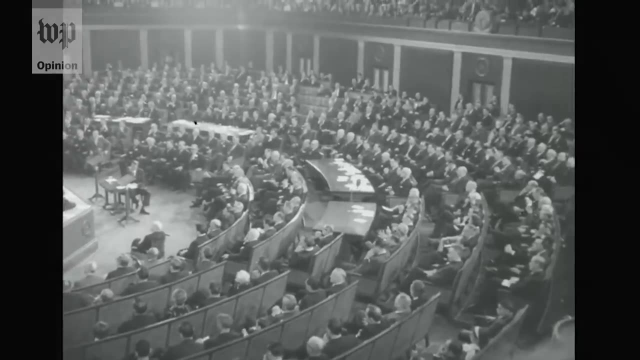 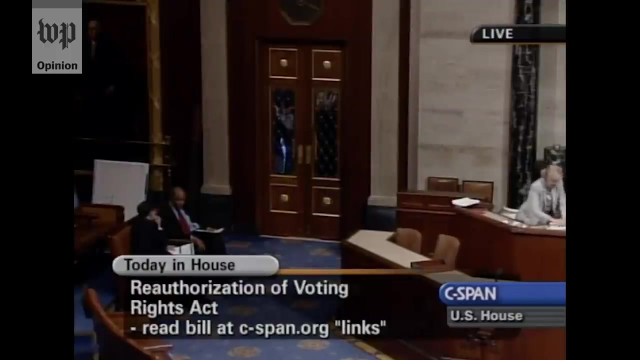 by requiring bilingual elections to vote. Congress reauthorized the Voting Rights Act in 1982,, 1992, and 2006.. The 2006 renewal included 15,000 pages of evidence of ongoing discrimination in voting. Congress said there was progress in eliminating 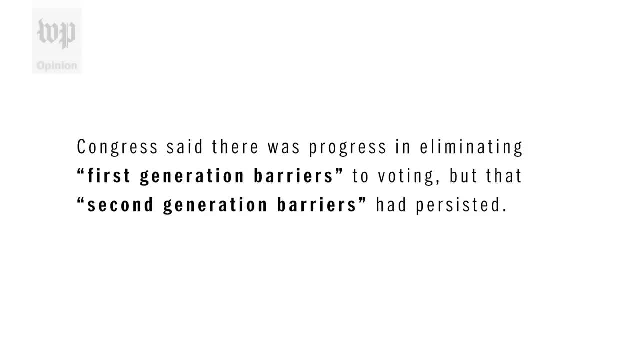 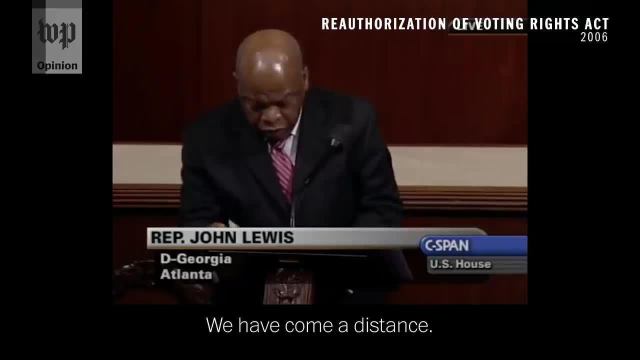 first-generation barriers to voting, but that second-generation barriers had persisted. Yes, we have made some progress. We have come a distance. We are no longer met with bull whips, fire hoses and violence when we attempt to register and vote. 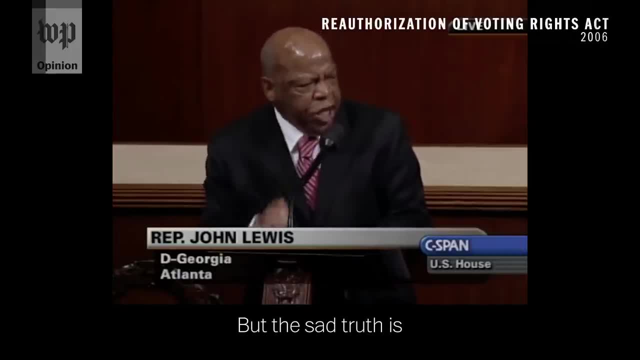 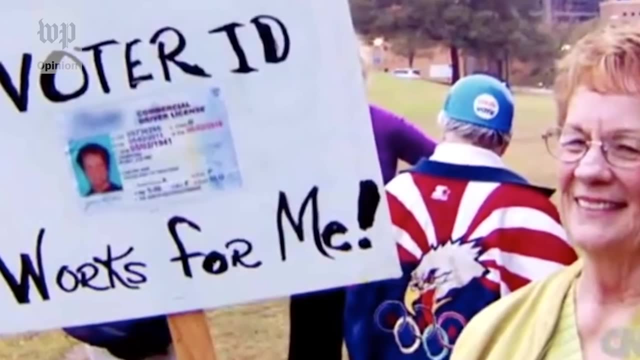 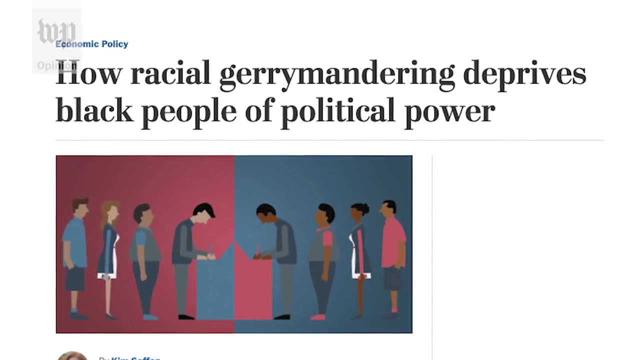 But the sad fact is. the sad truth is discrimination still exists. Second-generation barriers were laws that diluted the political power of minorities at the polls and included things like racial gerrymandering, poll closures, voter ID laws and cutting down early voting. 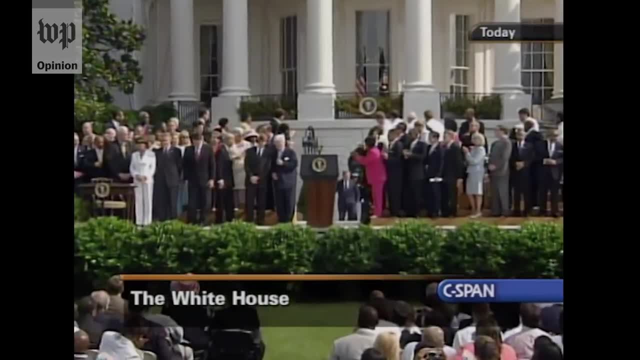 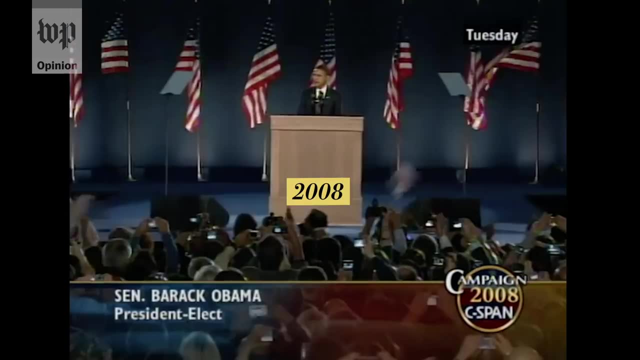 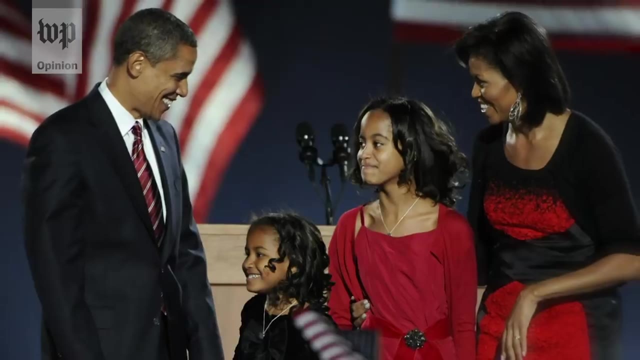 and same-day voter registration On a bipartisan basis, the Voting Rights Act was reauthorized for 25 years. Two years later, in 2008,, America elected its first Black president. The election of Barack Obama is one in the latest string of the advancement of Black folk. 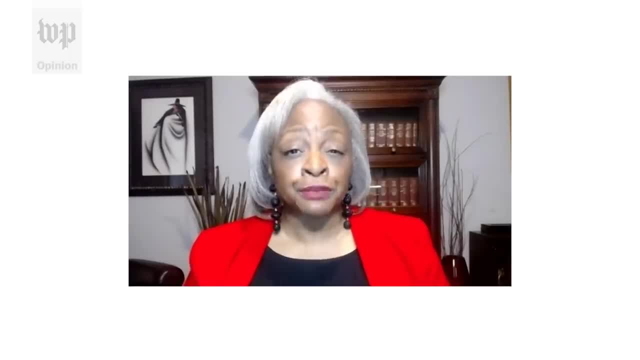 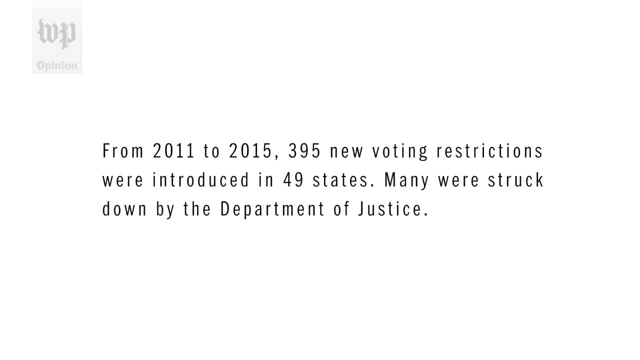 that leads to this incredible white rage. In 2010,, conservative Tea Party candidates swelled within the Republican Party. From 2011 to 2015, 395 new voting restrictions were introduced in 49 states, many of which were struck down. 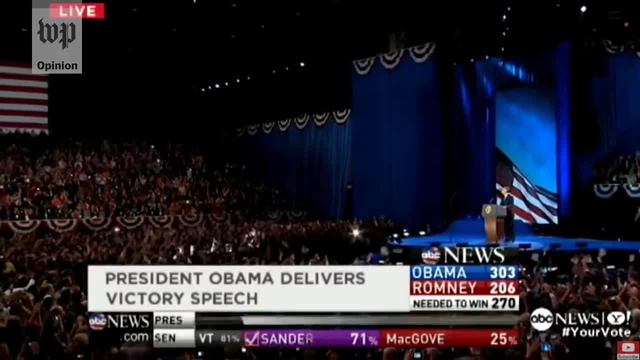 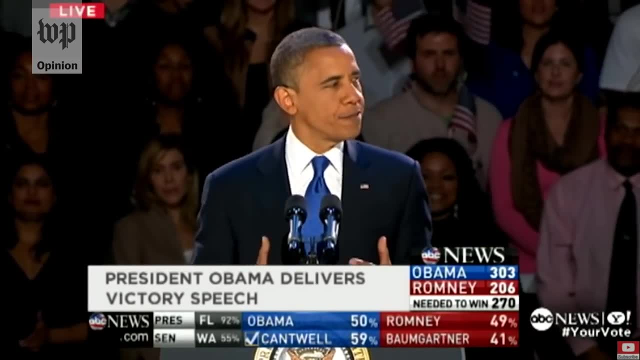 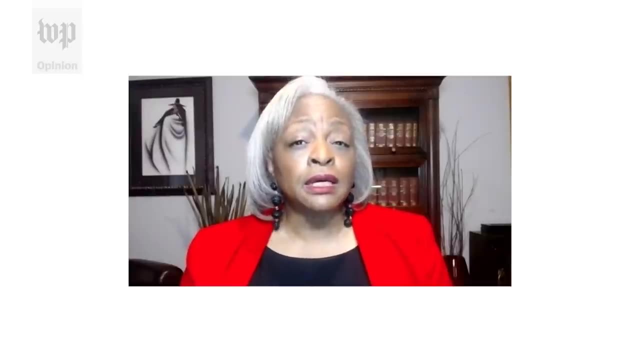 by the Department of Justice Anderson says the election and then re-election of America's first Black president was a factor behind the voting restrictions. His advancement was the penultimate advancement and therefore was the penultimate affront. I'm not surprised then that in his second term 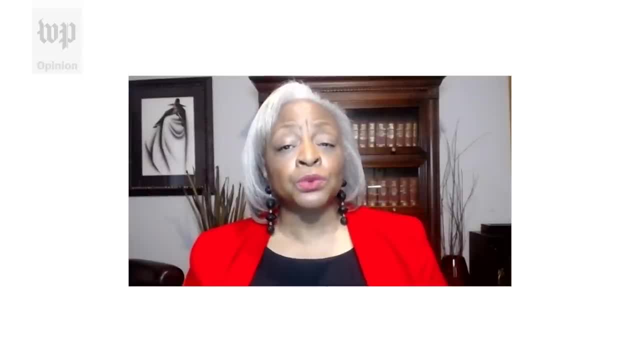 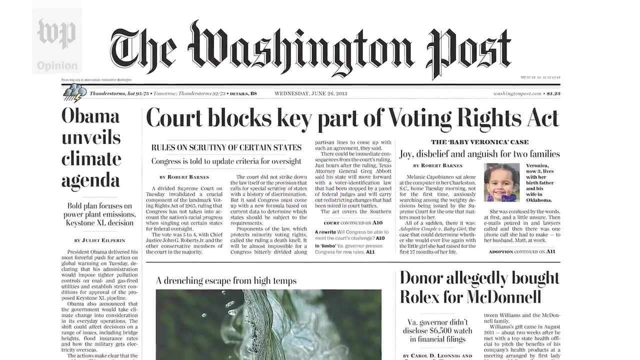 the US Supreme Court ruled in Shelby County v Holder that the Voting Rights Act, particularly Section 4, which was what they called their preclearance provision, the US Supreme Court gutted that The Shelby ruling released nine states. 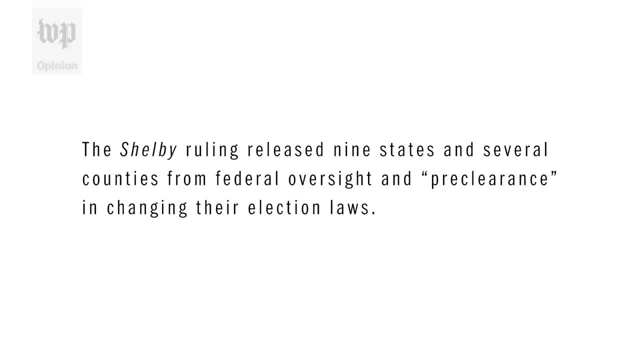 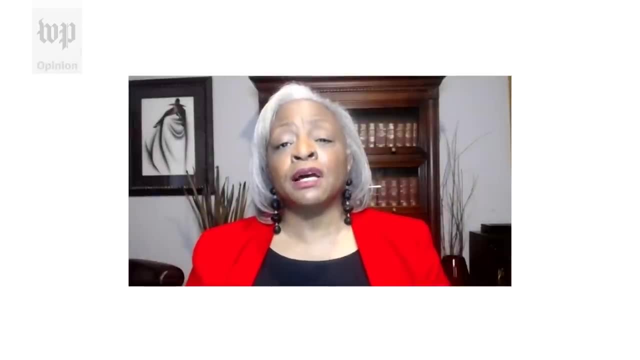 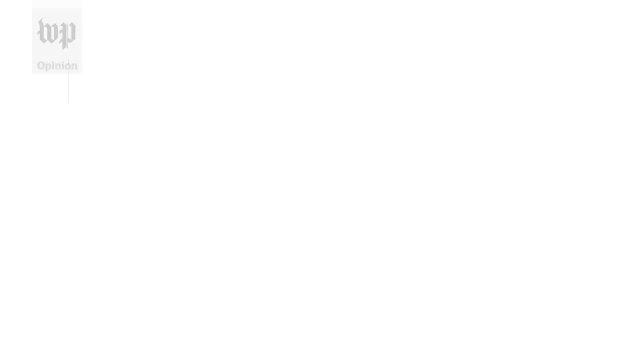 and several counties from federal oversight and preclearance in changing their election laws. Southern states reacted swiftly. Two hours after the Shelby County v Holder decision, Texas implemented its racist voter ID law. Two months later, North Carolina enacted HB 589,.